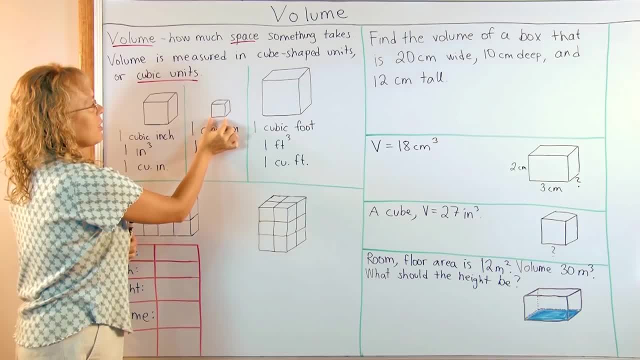 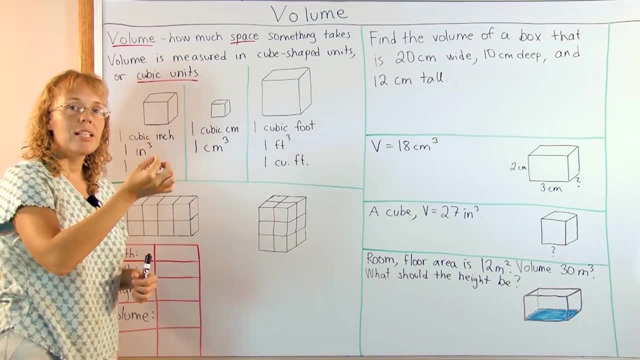 three times by itself. See here, this is centimetre by a centimetre by a centimetre. It's like centimetre times centimetre times centimetre. Centimetre multiplied by itself. Centimetre multiplied by itself three times. that's where that three comes from. 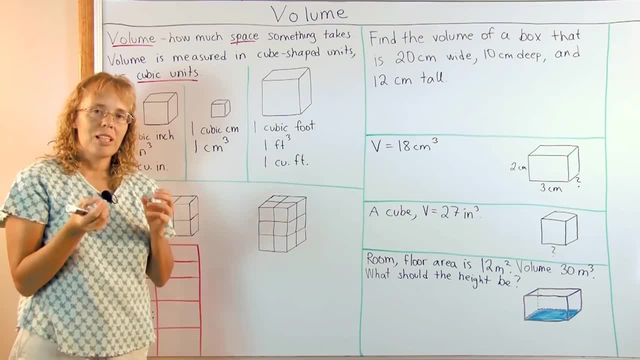 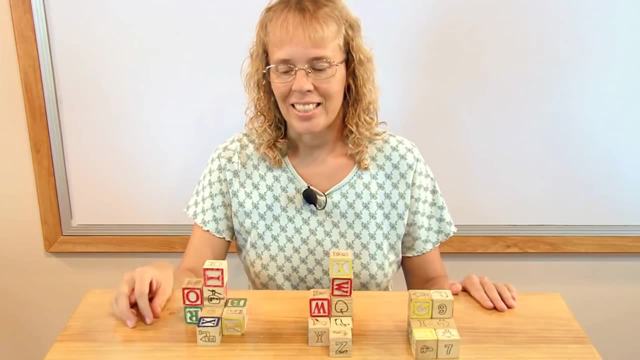 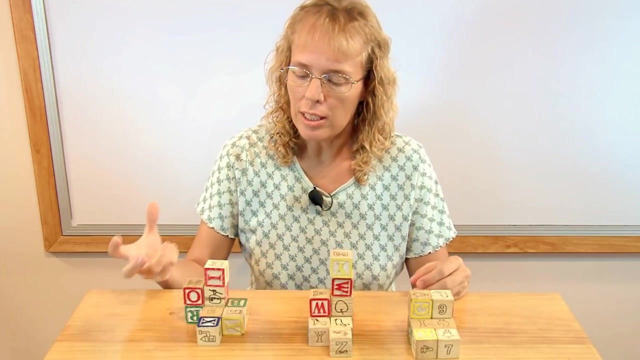 And children really need to use some manipulatives or some real blocks to understand some basic ideas about volume and cubic units. Like I said, children need to also play with blocks or unit cubes, if you have them, some kind of manipulatives, to get the feel for volume and how it is composed of cubic units. 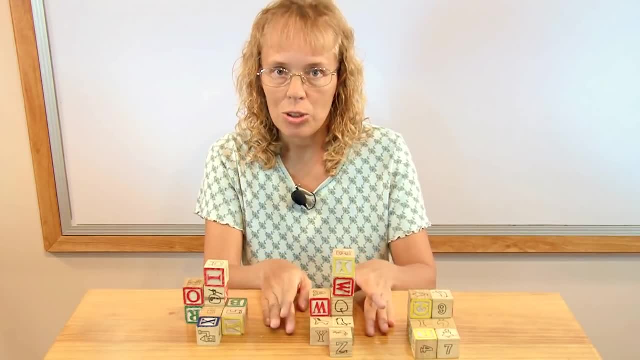 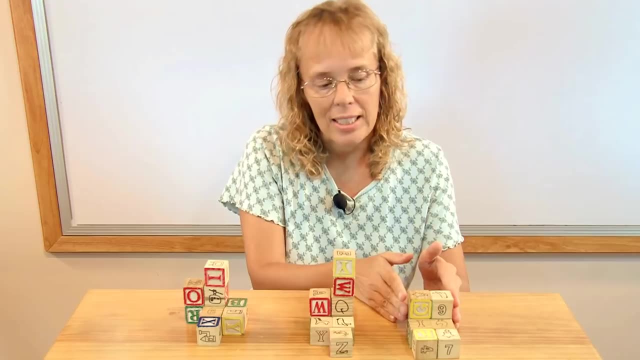 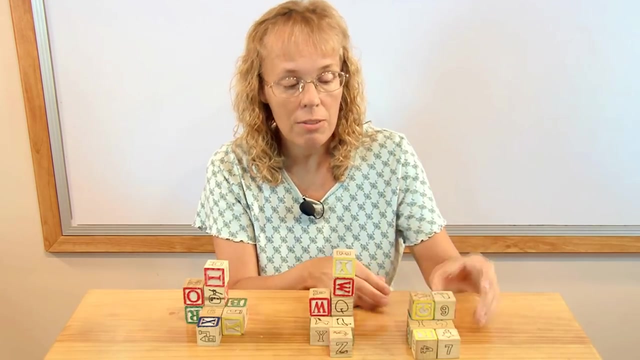 One type of exercise that school books always have is that children just need to count how many blocks are in some kind of set up, such as here or here. What is the volume of this thing? How many blocks are there? So we can see two here, two here, two at the top and two behind here, a total of eight. 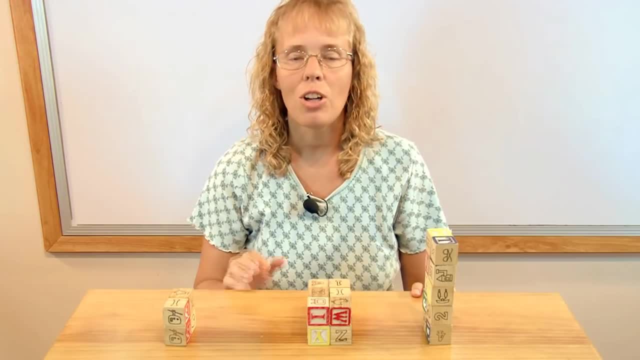 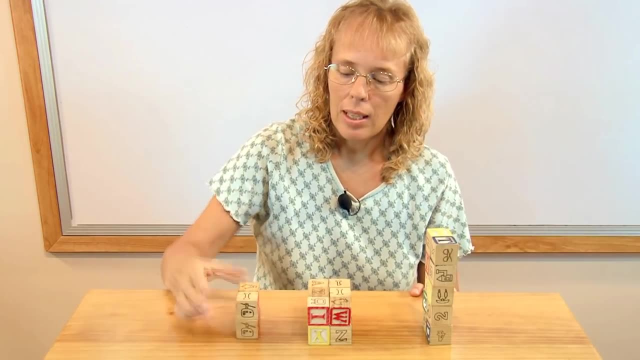 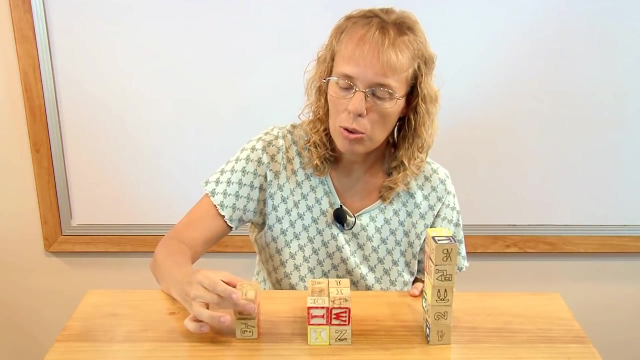 cubic units. Another thing children need to understand is the volume of a box or of a rectangular prism, And let's look at some examples here that I made. Basically, the idea here is that You can just, instead of counting the blocks one by one, you can just look how many are. 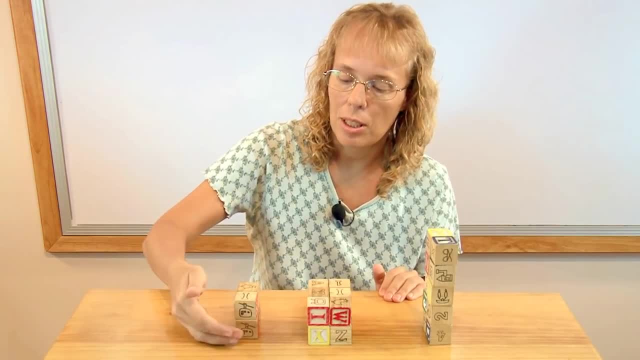 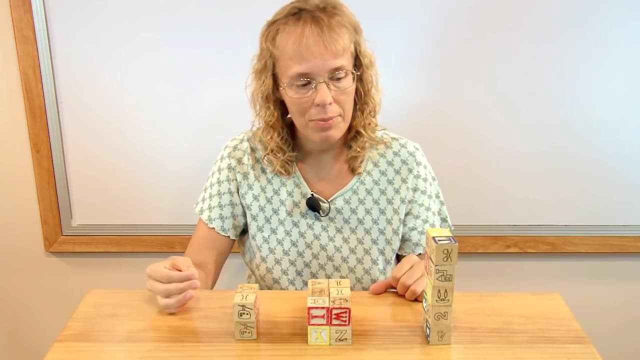 here on the bottom and then go that many times how many layers up it goes. There's two on the bottom and then two layers up in this one, so a total of four. right Here we have two on the bottom and then we have one, two, three, four, five layers up. 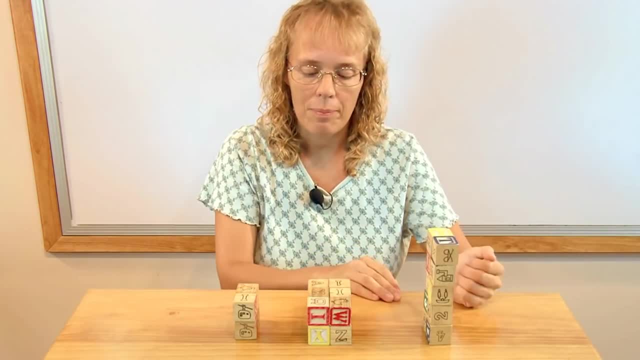 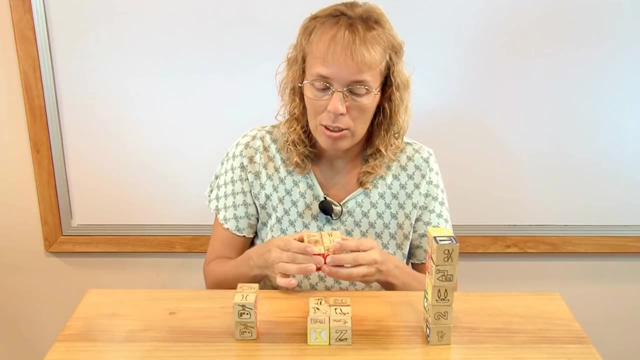 So five times two is ten blocks, ten cubic units in total. Or here you can look at the bottom, And even the bottom you can find out by multiplying. You can find how many blocks there are by multiplying two times three, right. 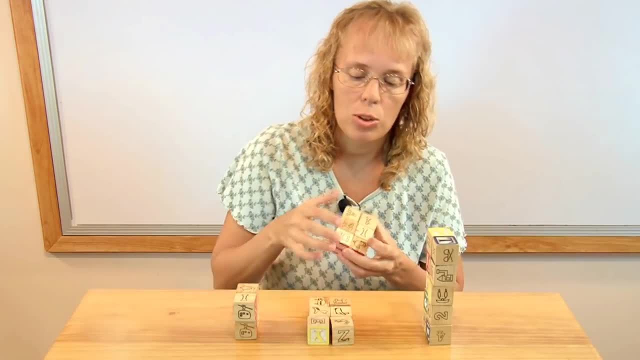 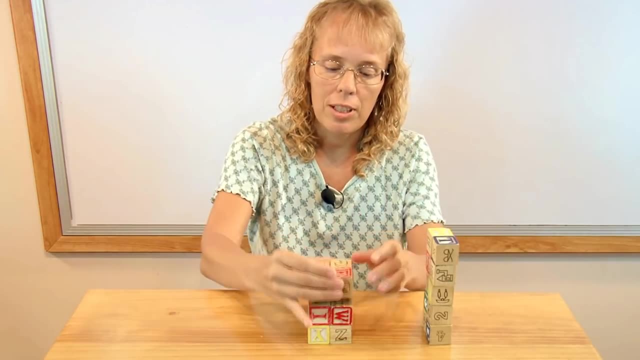 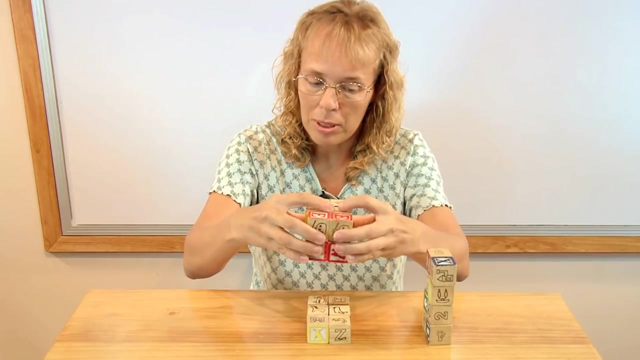 And that is your width and your depth. Width times depth: two times three is six, And then another layer of six. six times two is twelve. So even if I add here more, you can still see the same principle. We can look at the bottom and go two times three to find how many blocks on the bottom 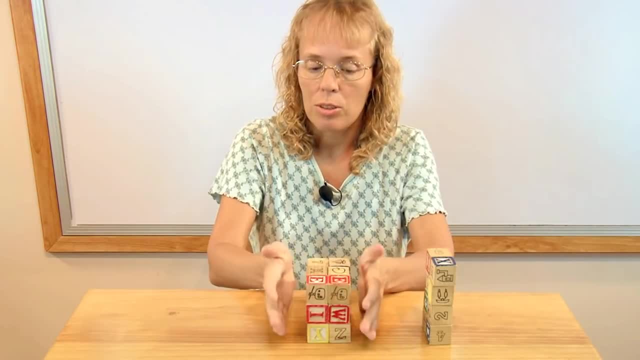 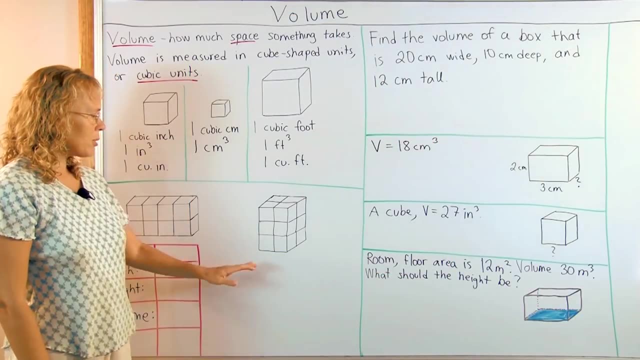 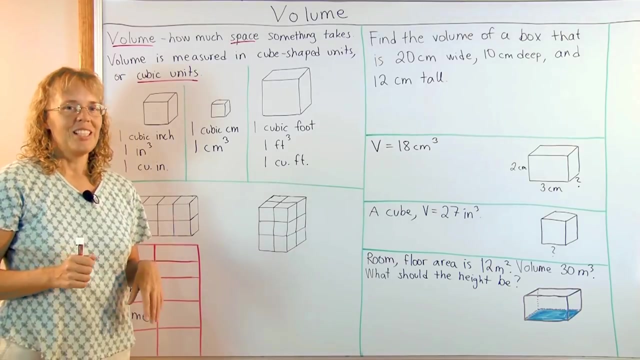 layer. That times three the height to get the total volume of this rectangular prism. Now let's look at a few problems. where we have a box or a rectangular prism, it's called, But in third or fourth grade you can call it a box. 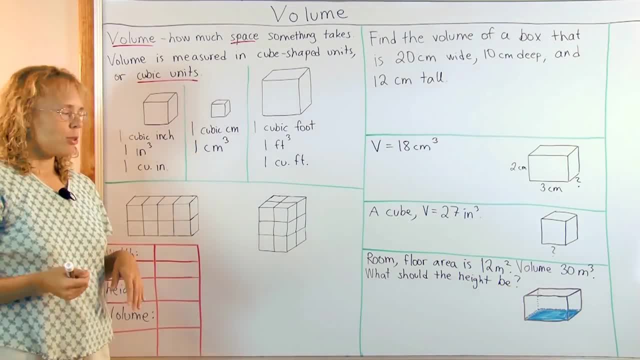 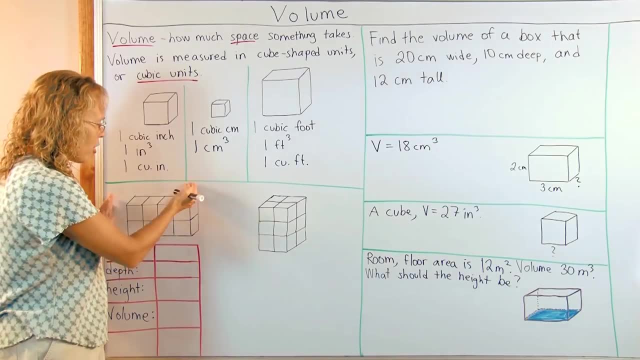 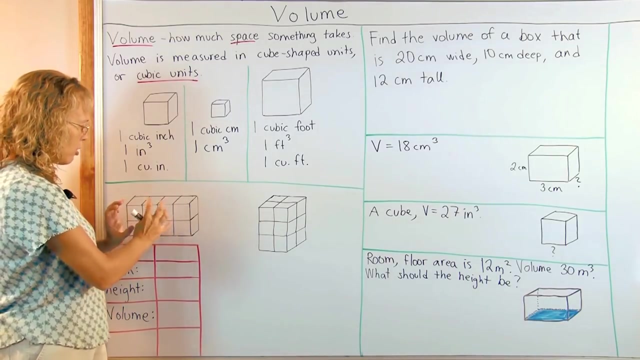 It's simpler And we have to find its volume. As we already saw with the blocks, you can simply use multiplication to find the volume of a rectangular prism or box. So let's say I have this many blocks stacked together into a box-shaped thingy. 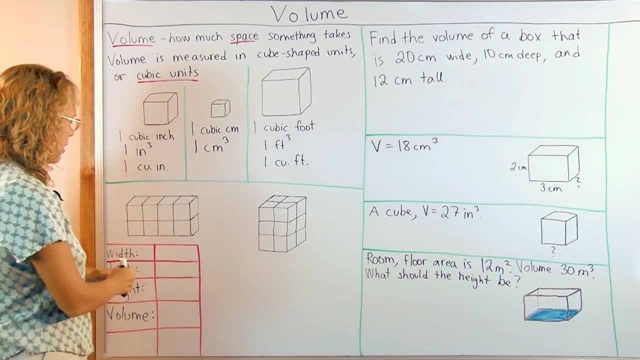 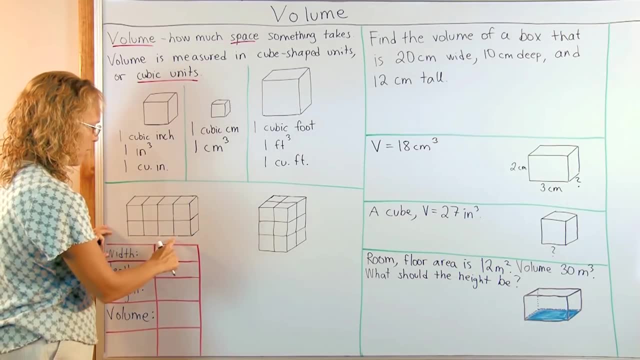 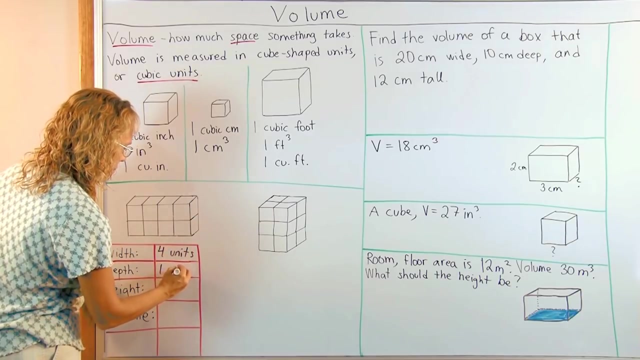 I want to find its volume. I can use multiplication. I can check how wide it is. How many units wide is this? Okay, it is one, two, three, four, Four units wide. And how deep is it? It's just one unit deep. 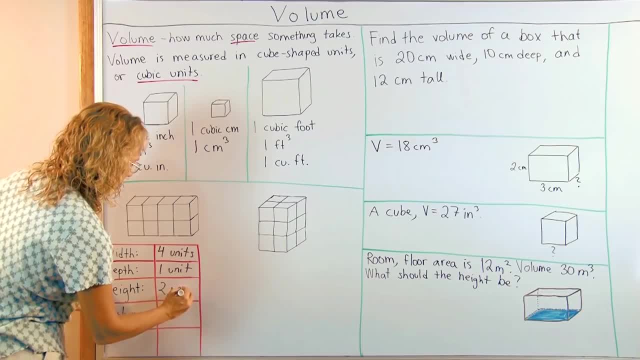 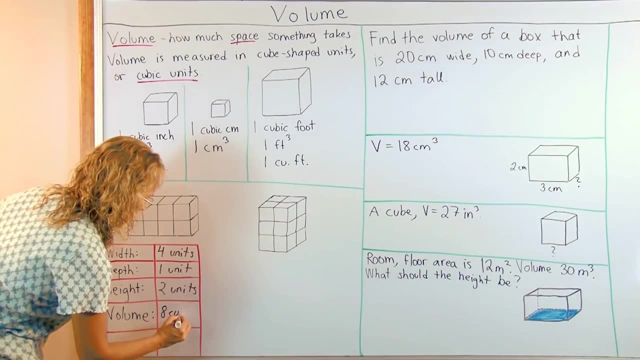 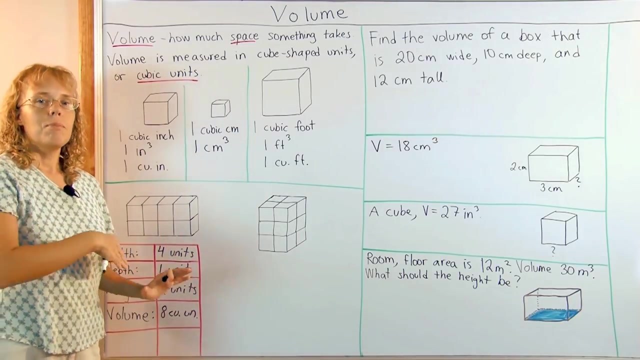 And how high is it? Two units high. And then I multiply four times one times two, I get eight cubic units cubic and units as its volume. Okay, And here I didn't have any measurement unit to use. I didn't say that these are centimeters or feet or inches, but I just used a generic. 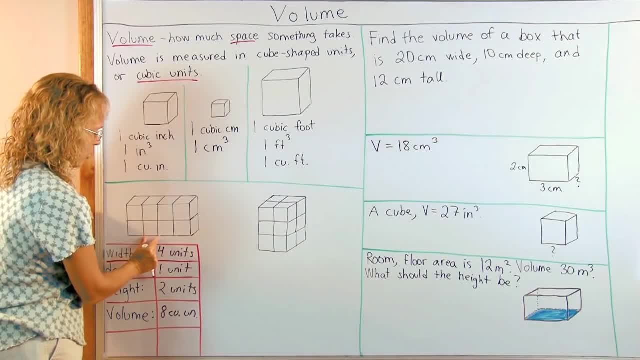 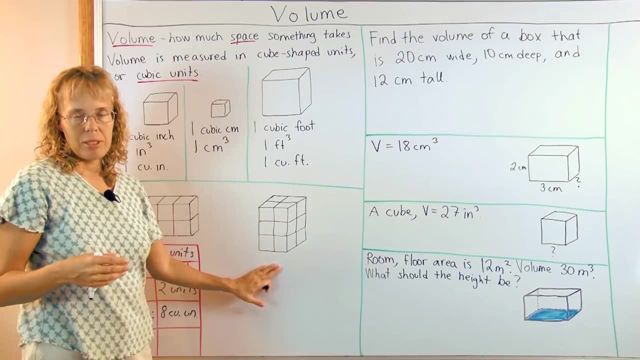 term units. So that's why the length is just a unit and then the whole volume will be cubic units. But here let's say that the length is just a unit and then the whole volume will be cubic units. So let's say that we are using centimeters as a basic unit. 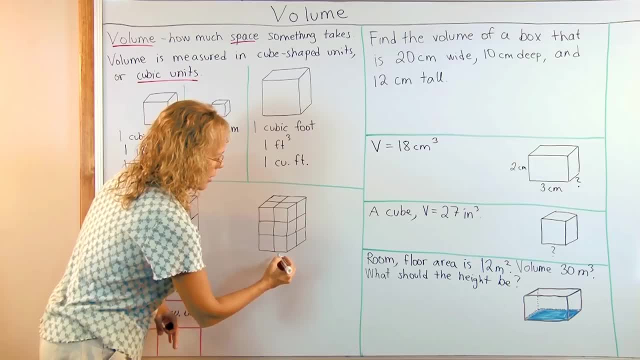 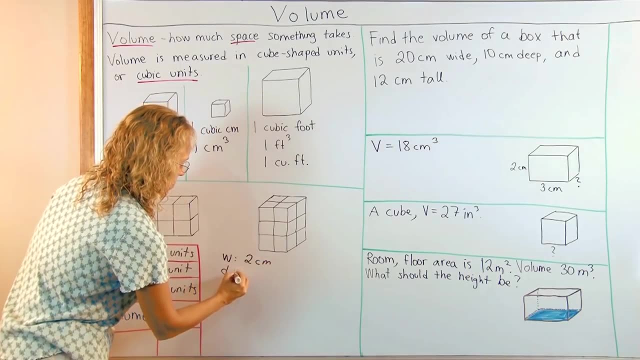 So here would be this width would be exactly two centimeters, and let me write it here: Width, two centimeters, And then depth: How deep is it this way? Two centimeters, And how high is it? Three centimeters. 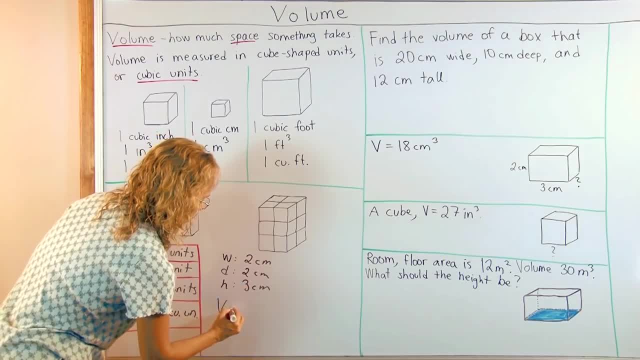 Height is three centimeters, Then we're going to get volume- This big V is volume- By multiplying Two times two times three, which is four times three, And then we're going to get volume- This big V is volume Four times three. 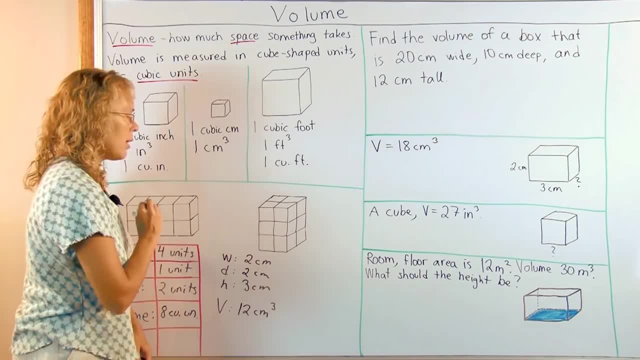 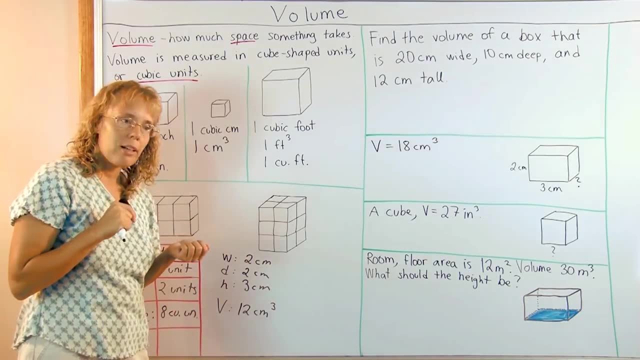 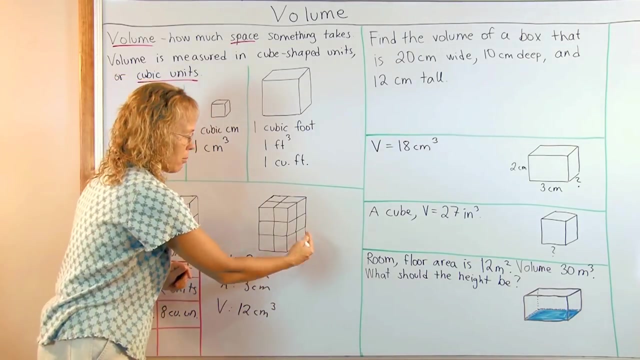 Twelve, Twelve cubic centimeters And, like you saw, with the blocks, you can also think of this multiplication this way. Think first of the bottom layer of this whole thing. In the bottom there's two blocks times two blocks. There's just four blocks on the bottom right. 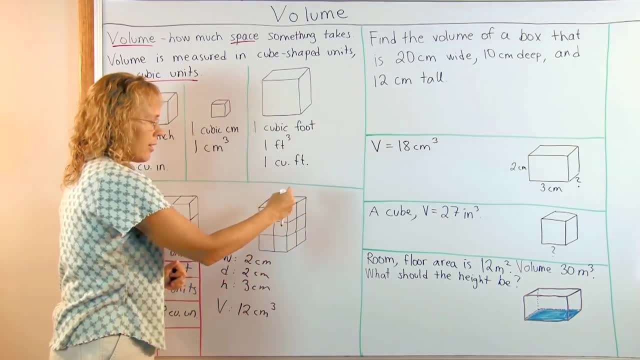 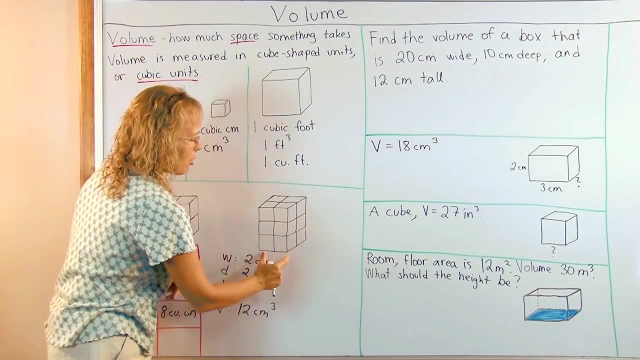 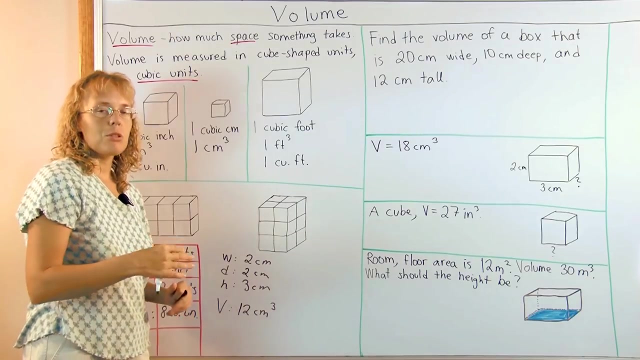 And then you'd think of how many layers high it is. in blocks There's actually three layers or three levels. So four times three The blocks on the bottom times how many layers you have. Four times three equals twelve. So there's twelve cubes here. 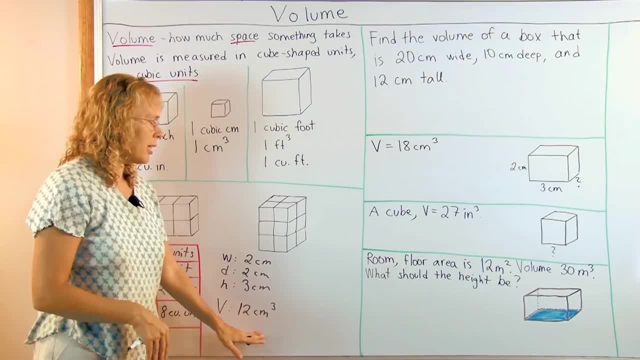 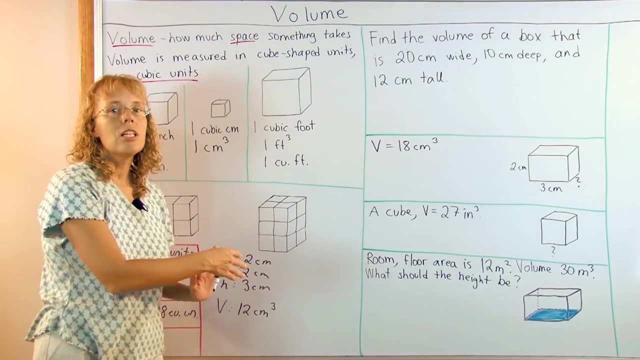 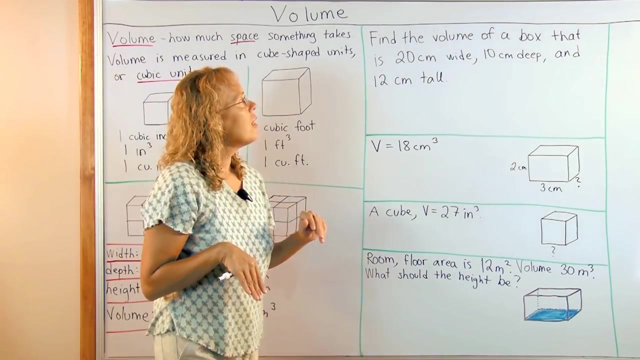 And the volume is twelve cubic centimeters. After children understand this idea, how to calculate the volume by multiplication and how it consists of these individual little blocks, then they're ready for other word problems. Here's one: Find the volume of a box that is twenty centimeters wide, ten centimeters deep and four times 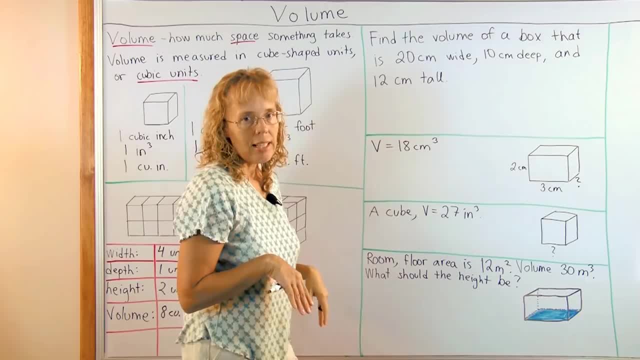 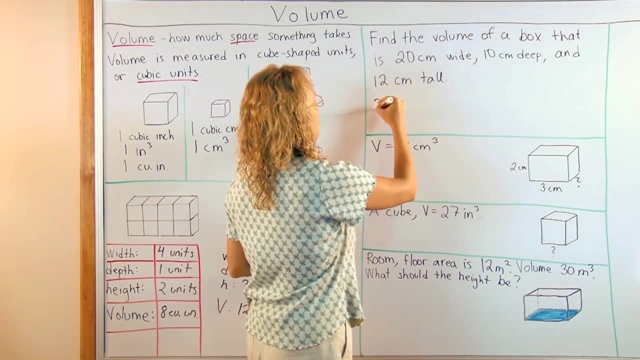 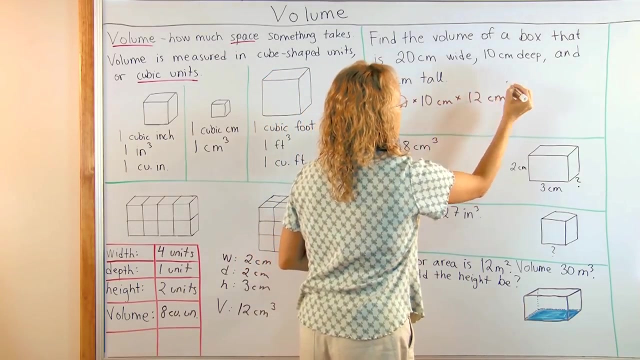 three is twelve. This is exactly the same situation as I have here. We simply need to multiply those three numbers. So let's go twenty centimeters times ten centimeters times twelve centimeters, And to multiply these three numbers where there's zeroes here involved, you can first: 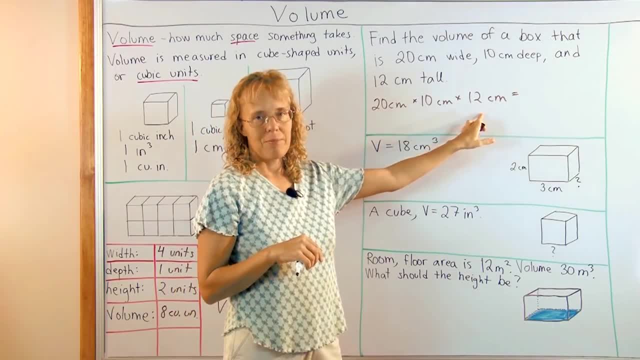 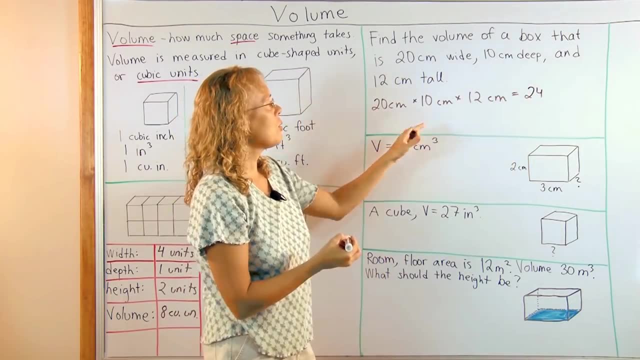 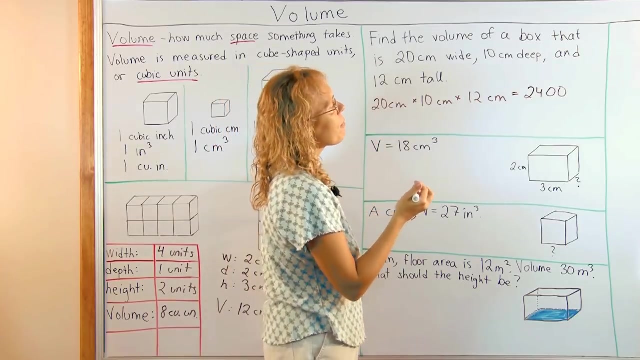 ignore the zeroes and multiply two times one times twelve, which is just two times twelve. right, Then you tag however many zeros you had here, One and two. Tag the zeros there. That's like a little shortcut for multiplying by 10 or 20 or whatever. So 2400, and then our centimeter. 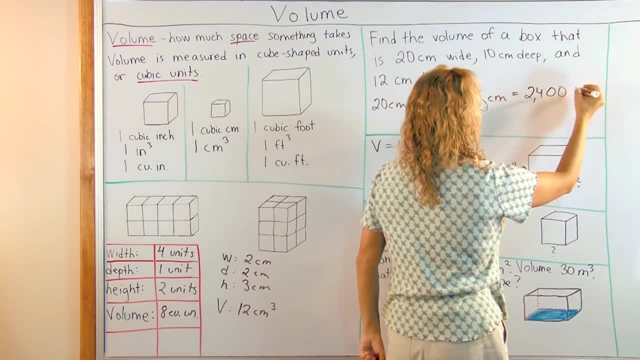 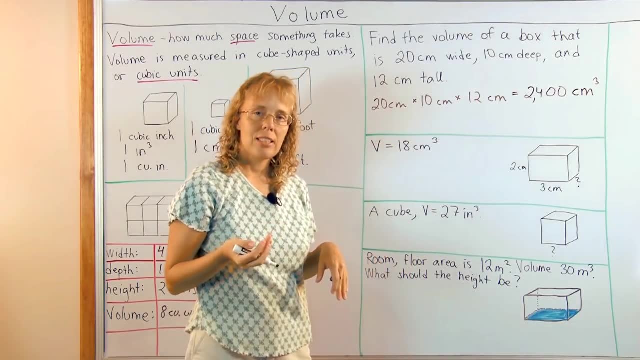 got multiplied by itself three times. so we get the cubic centimeters here. You know, centimeter cubed, like that. Here's another word problem. but this time we are not asked the volume, because we already know the volume. The volume is given here and it is asking: 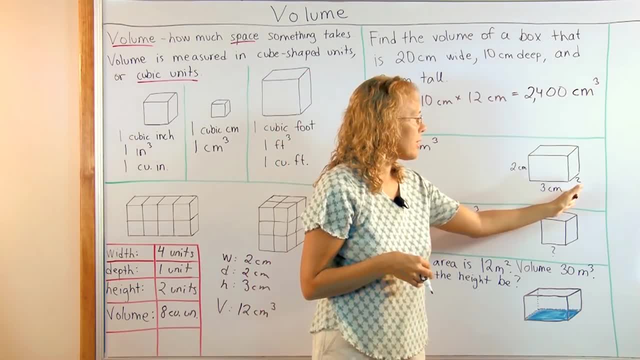 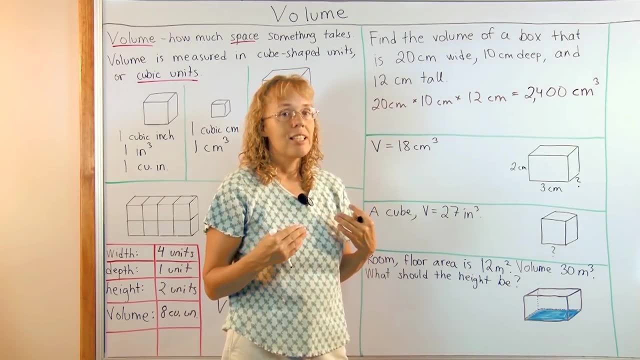 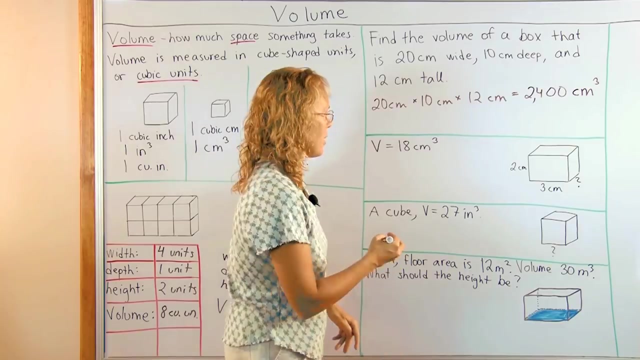 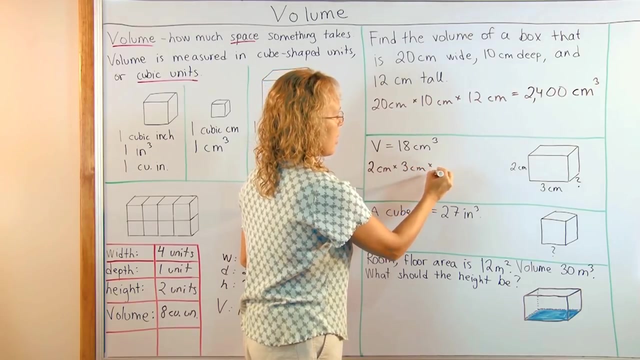 how deep is this box? It is two centimeters high, three centimeters wide. How deep is it? And this time we need to think of multiplication again, but this way: Two times, three times, this number is 18, right, Let me write here: two centimeters times, three centimeters times. 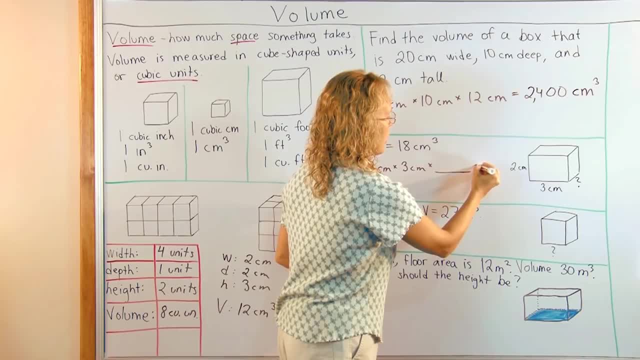 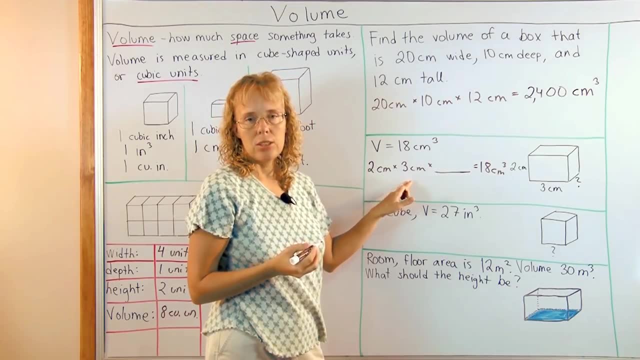 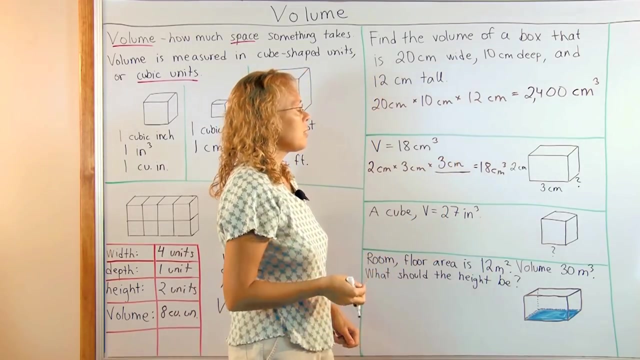 18.. And the depth that we don't know? that has to equal 18 cubic centimeters. So simply, two times three is six, and so six times what is 18?? The answer is three centimeters. Okay, so it's an easy problem in that sense, but children need to notice that it is not asking. 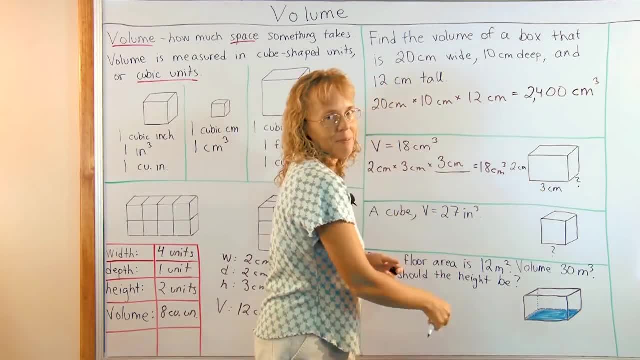 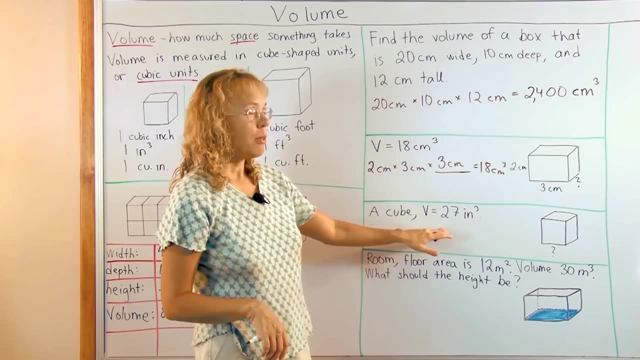 for the volume. You do not multiply 18 times two times three, But you think in reverse, so to speak. This is a similar one, Similar problem Again. we are given the volume, We are not being asked what the volume is, So we cannot. 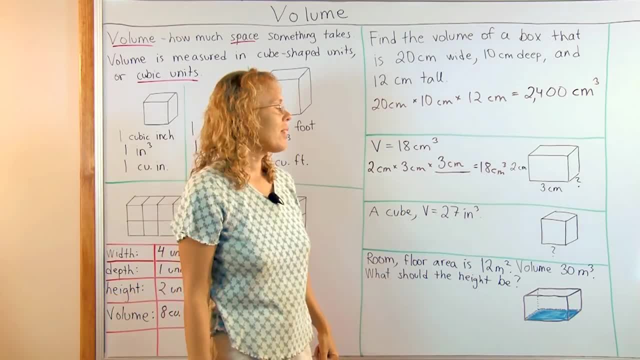 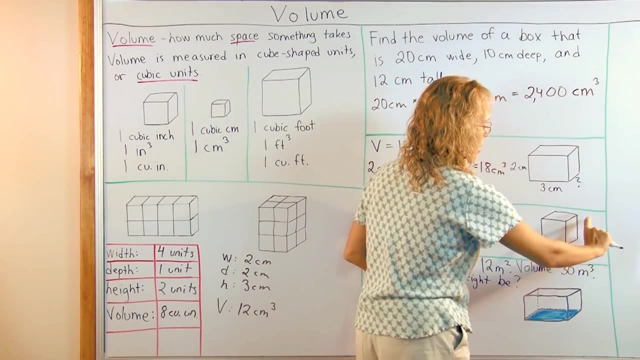 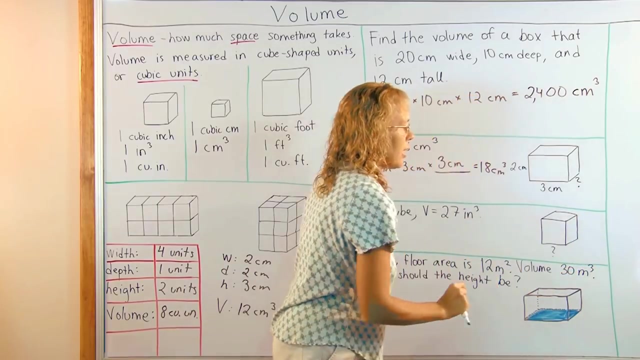 go multiplying 27 times 27 times 27.. And it is a cube. Now. that means that the width and the depth and the height are equal. It's going to be the same number, Whatever number is here. that number times itself, times itself, gives us 27.. And here children can use guess. 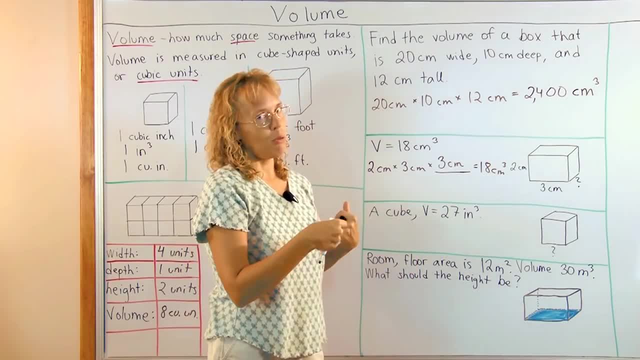 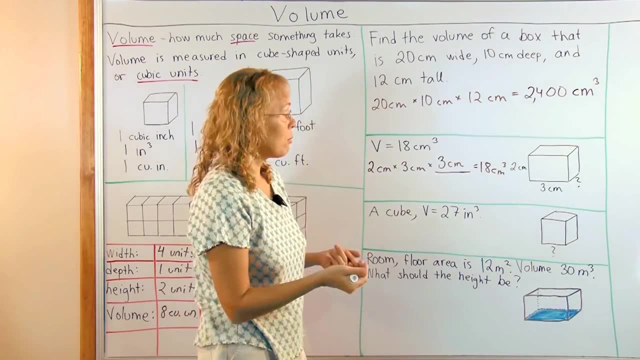 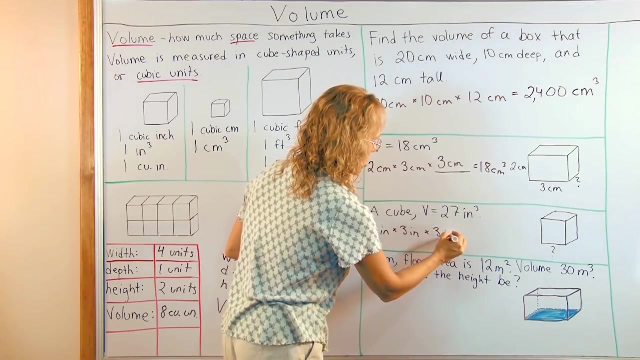 and check. Okay, You know, one times one times one, One times one times one, One times one won't work right. Two times two times two won't work either. But three times three times three will work. We will get three inches times three, inches times three inches equals. 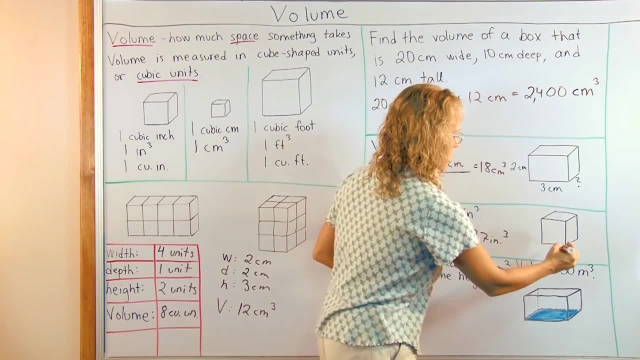 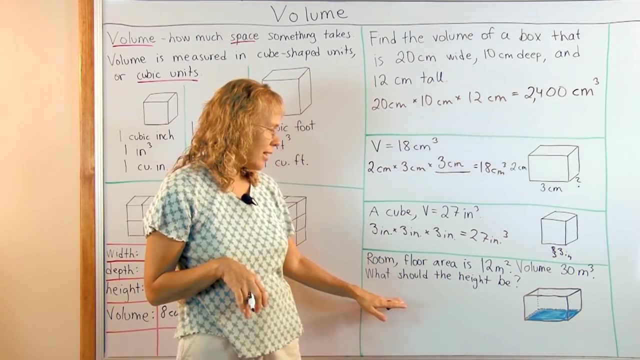 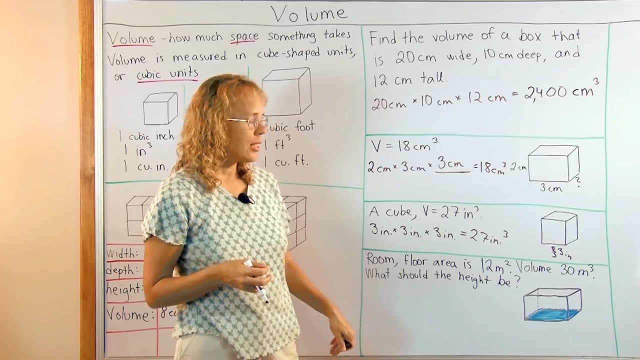 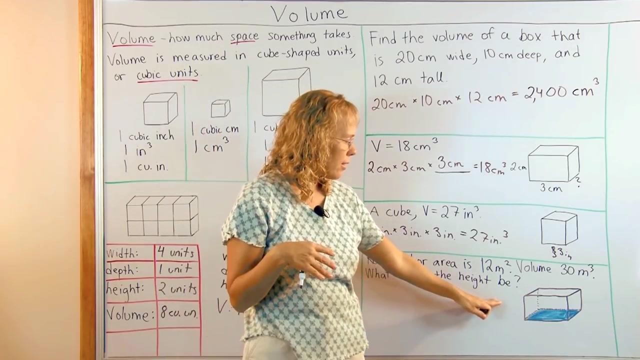 27 cubic inches. So this here is three inches. And lastly, a problem that again is not asking for the volume. It is a little different from these two, again, because it does not give us the width, the height, the depth. It doesn't give us those numbers, It's asking for the height. What? 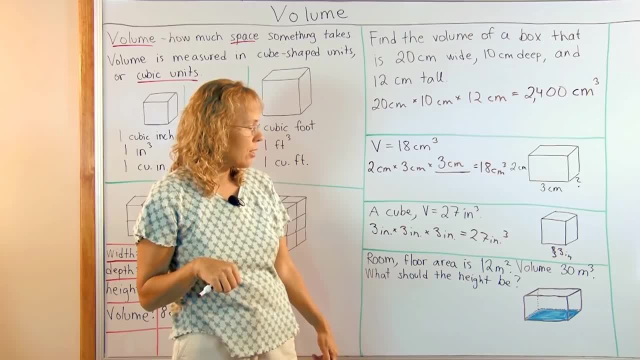 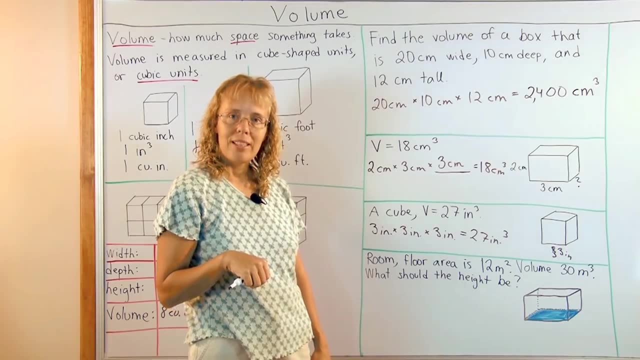 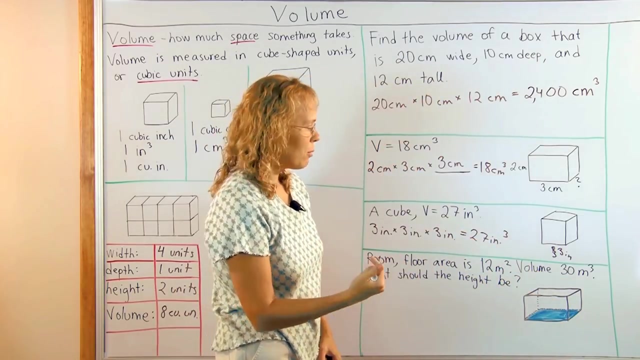 should the height be of this room? And it's not giving us the width or anything else, It's giving us the area. So how do we go about that now? To find the volume. I mean, we are given the volume, but to calculate the volume we would. 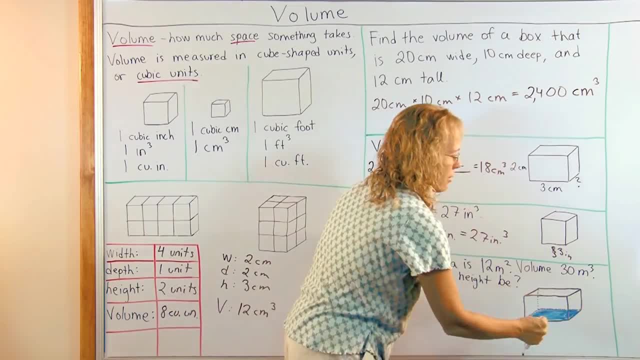 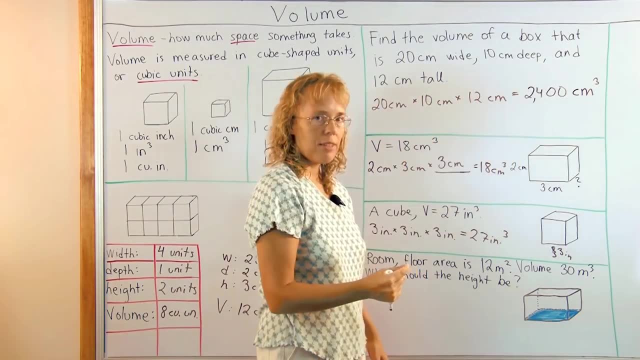 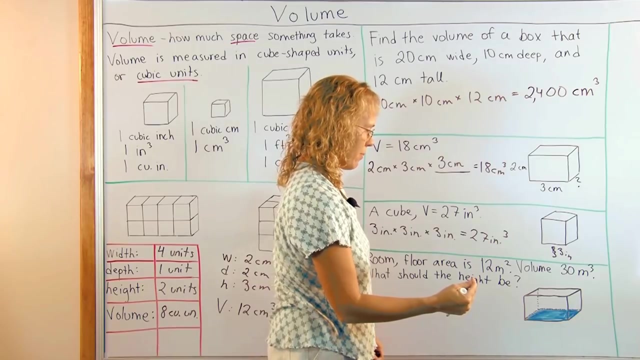 multiply this times, this times this right, And to calculate area, you would multiply this times this and the area is given. We know the floor area is 12 square meters, So this times this is 12.. We already know that. 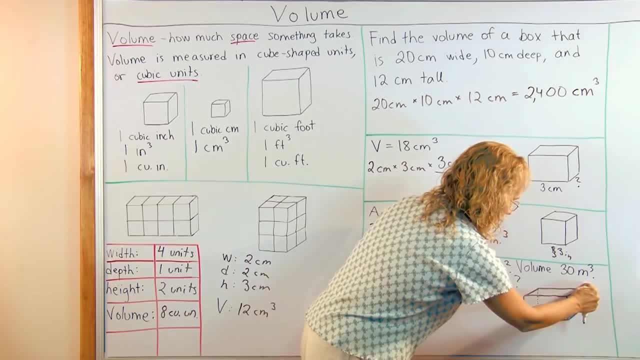 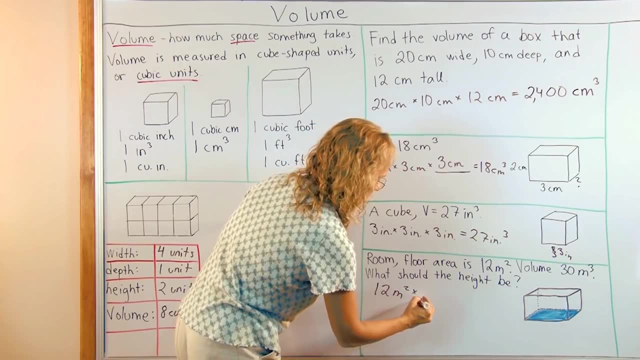 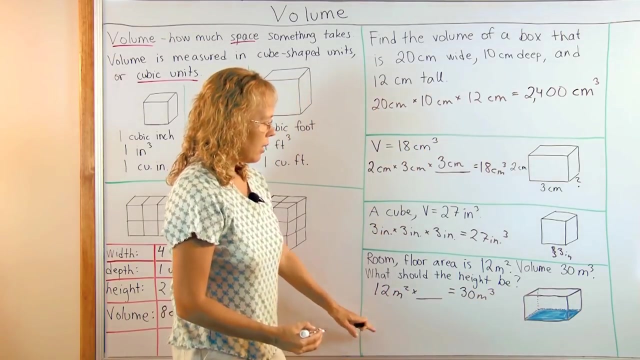 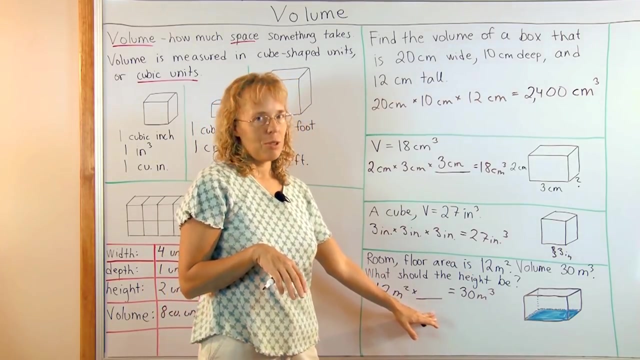 So therefore, the question is basically: 12 times that is 30.. We will get 12 square meters here. times something, Okay, something which is the height equals 30 cubic meters, the volume, okay. And to solve this you can again use guessing. check, Let me guess 12 times 2, 24.. That won't work.